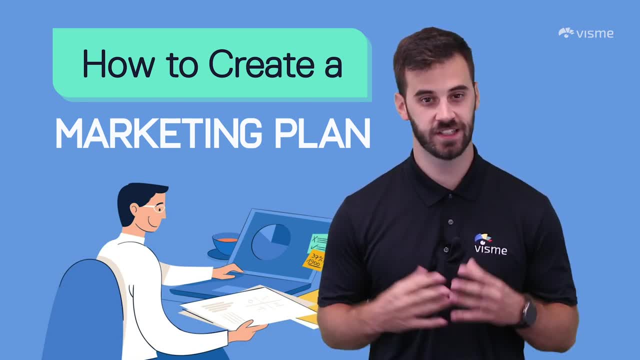 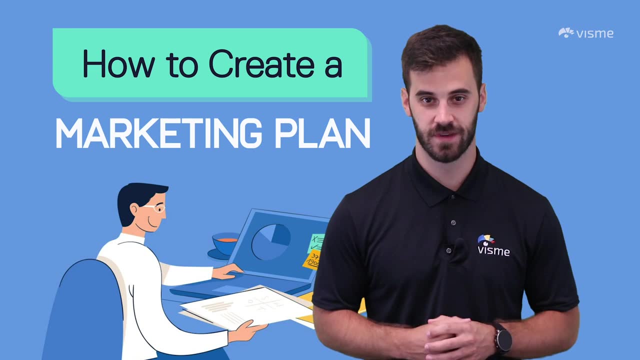 a marketing plan, and these are extremely helpful when it comes to understanding your business, clarifying your goals, staying focused and keeping everyone on your team on the same page. In this video, I'll take you through the 7 necessary steps to creating a winning marketing. 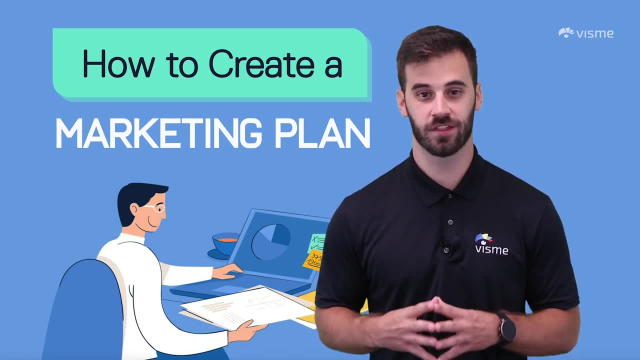 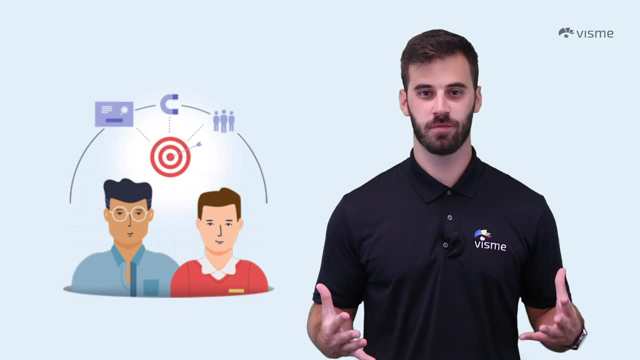 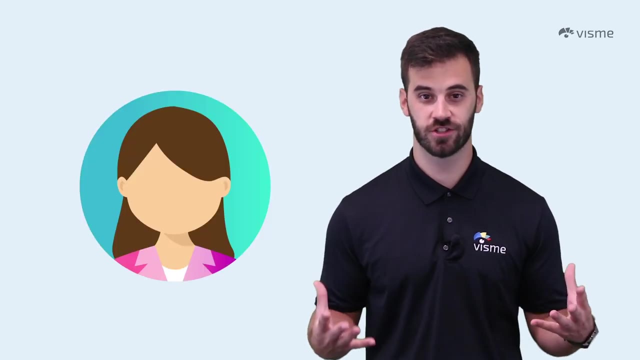 plan, as well as share a number of templates you can start with. Let's start with right away, shall we? Understanding the purpose behind a marketing plan is step number one. Ideally, it should be used to help you set your goals, understand your target audience and optimize the impact of your marketing. 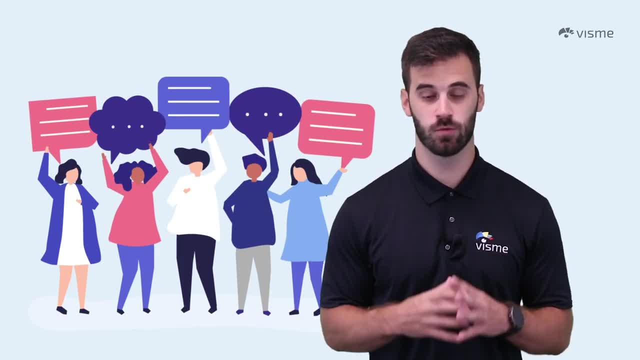 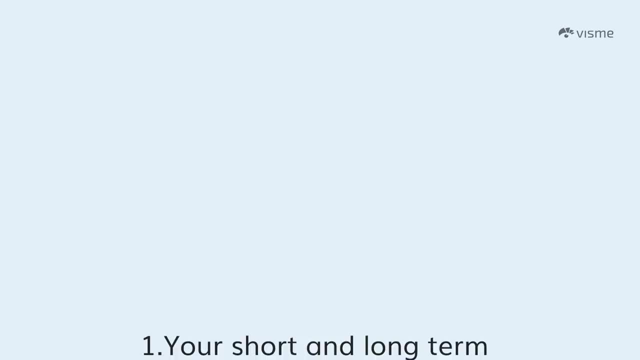 campaigns. Communicating your big strategy or idea is what your marketing plan is all about. In order to do this, every marketing plan should consist of the following: Number one: you are short in long-term marketing goals. Number two: a description of your target audience and their 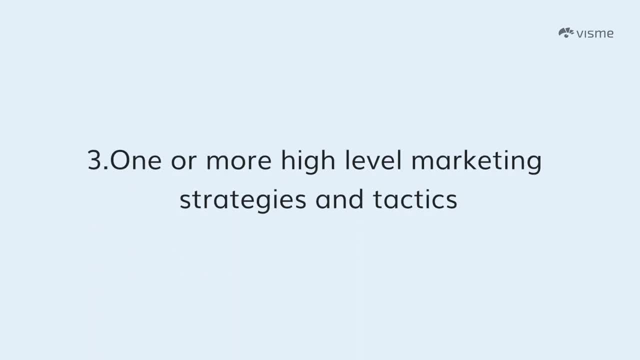 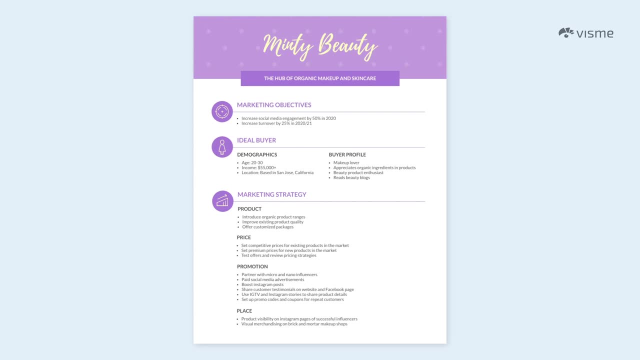 persona. And number three, one or more high-level marketing strategies and tactics. This infographic template, available on VizMe right now, features each of these key details. It clarifies the objectives, the target audience and strategies in an easily consumable page. If you wanted to go the. 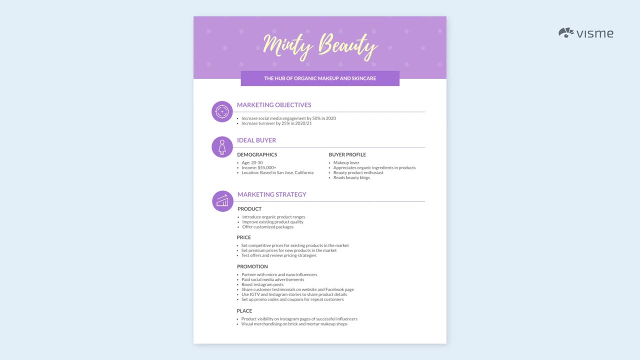 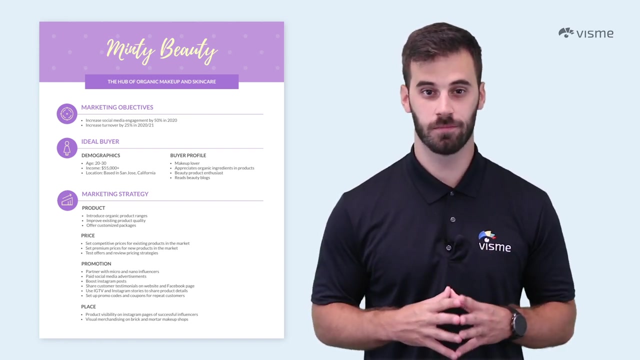 extra mile and include more detail. you could also add an overview of the current market situation, key performance indicators, budget or financial considerations or a timeline on when the plan will be carried out. Typically, all of this information is communicated on a PDF, just like the one we just saw, But if you're feeling creative, 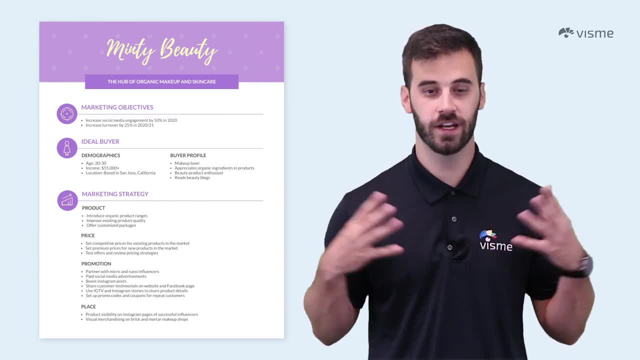 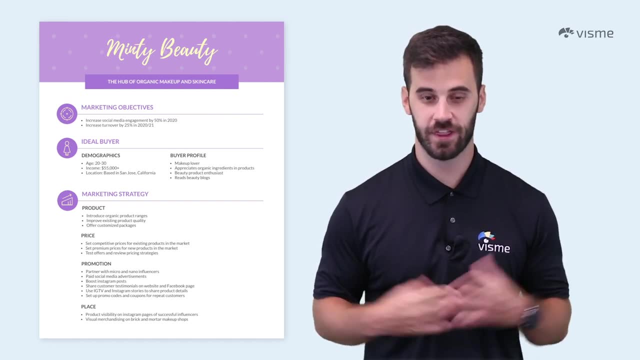 try creating an infographic, a full presentation or an interactive web page to share your plan. Who knows, It could be the difference between your plan and someone else's. Without further ado, let's dive into seven steps for creating an effective marketing plan. 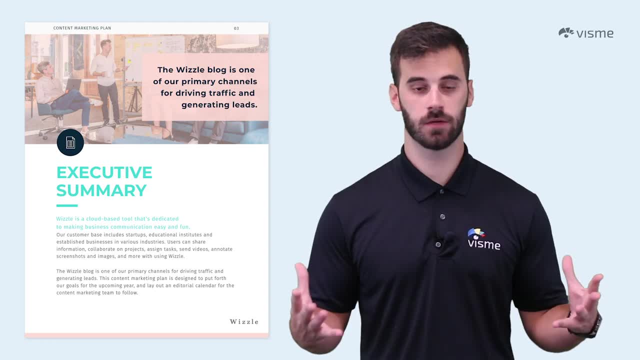 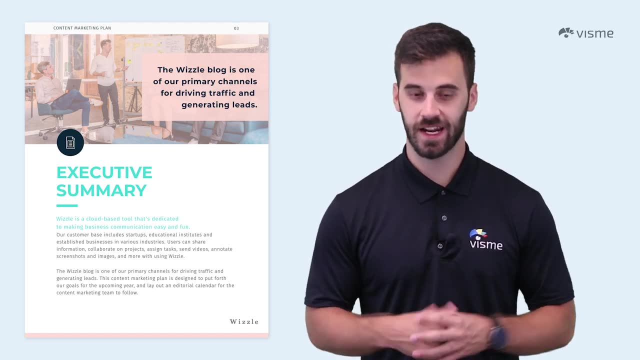 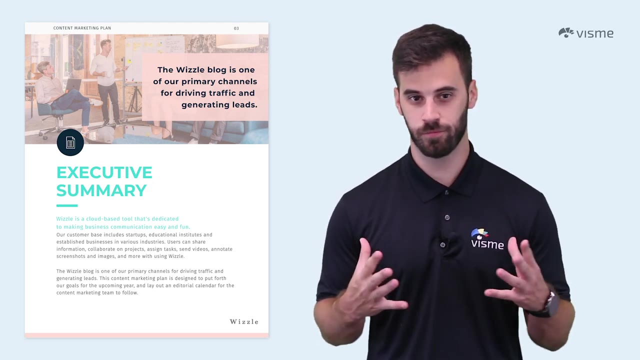 Step number one: start with an executive summary. This is essentially a brief summary or overview of your entire company and the key details of your marketing plan. It highlights the function of your business and the purpose of your plan. This shouldn't be very long. The summary can include past. 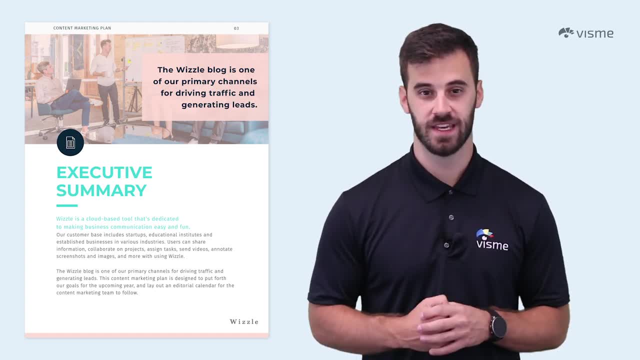 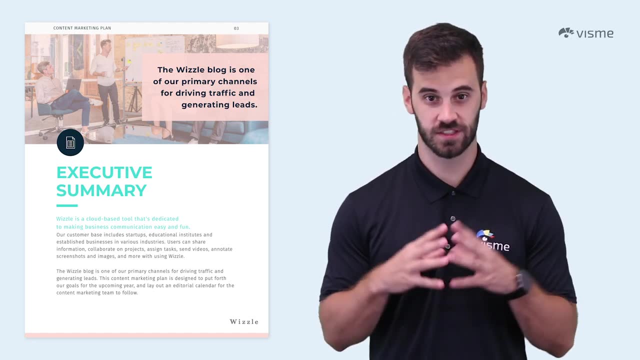 achievements and the future direction of the company. Consider this template. here. The details are concise and to the point. You want to tease your viewers on what's to come and get them on the edge of their seats. It's not overwhelming. just a quick introduction before you get into the meat. 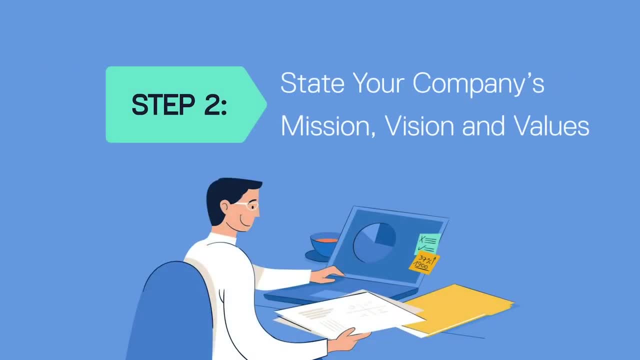 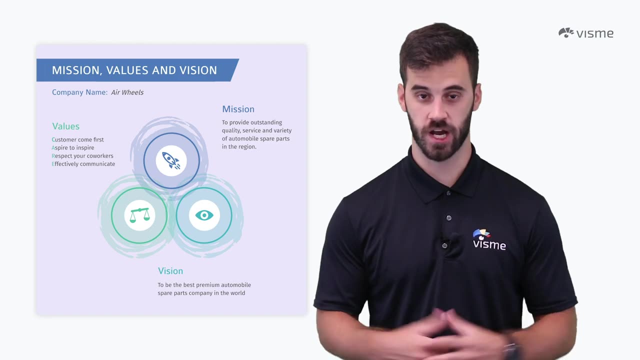 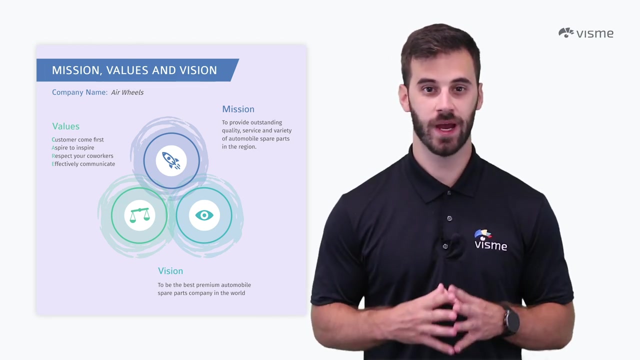 of your plan, Revisiting your company's mission, vision and values is important to highlight early on Why It'll provide clarity and answer any questions as to why your marketing plan is the way that it is. It'll show viewers. you had this in mind throughout your entire planning. 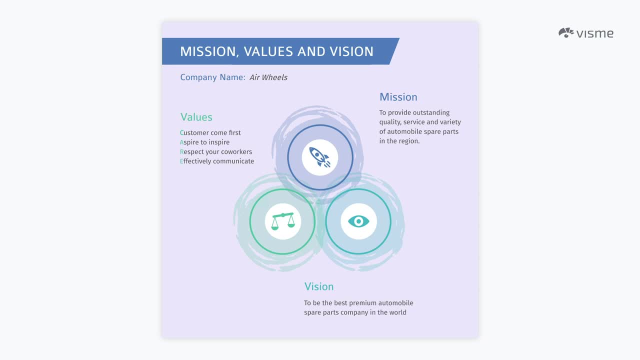 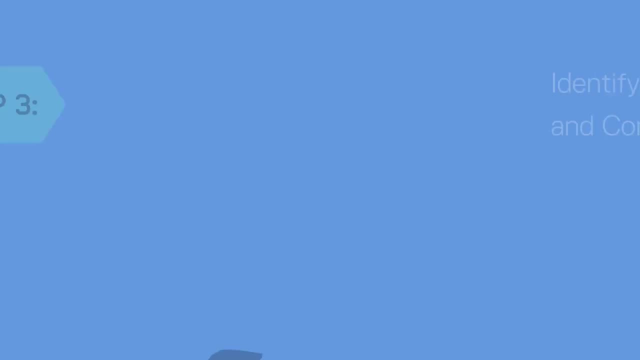 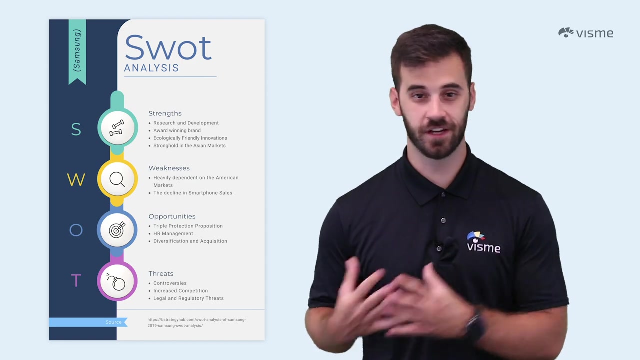 process. Templates like this can help because it'll educate or remind your viewers how your company got to the point they're currently at and where you're looking to be in the future. One of the first steps with any plan is doing your research: Study, the market study, the 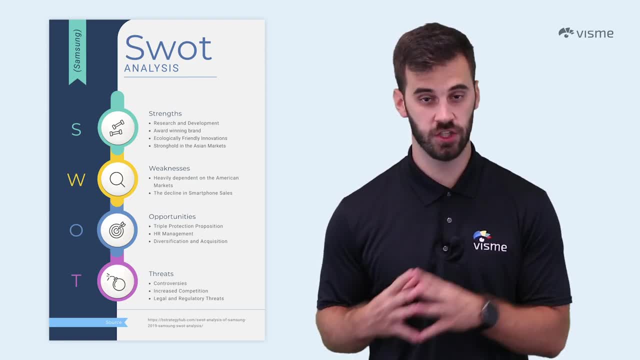 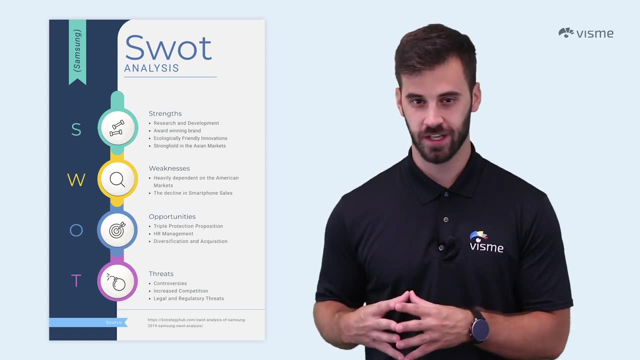 competition. What are others doing that's working, And then what can you do to make it even better? Deeply analyze your own company's strengths and weaknesses. Touch on what you're doing well, but don't be afraid to do it. Don't be afraid to communicate what you think could be stronger. A SWOT analysis or strengths. 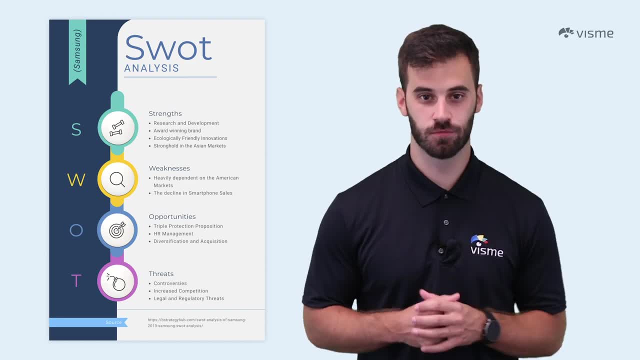 weaknesses, opportunities and threats is a great way to present your research. You can visualize the company's path, identify opportunities, set goals and so much more. This template right next to me can be edited in Visme and is completely customizable, From the text content to the colors. 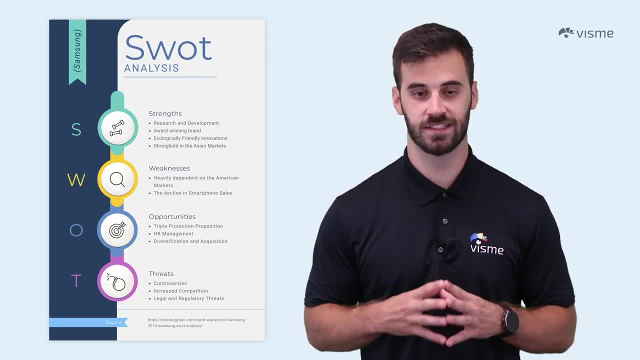 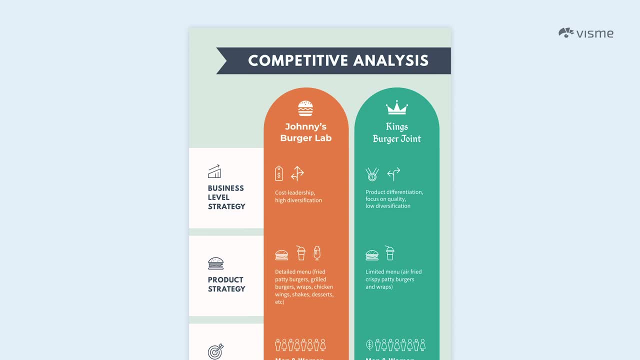 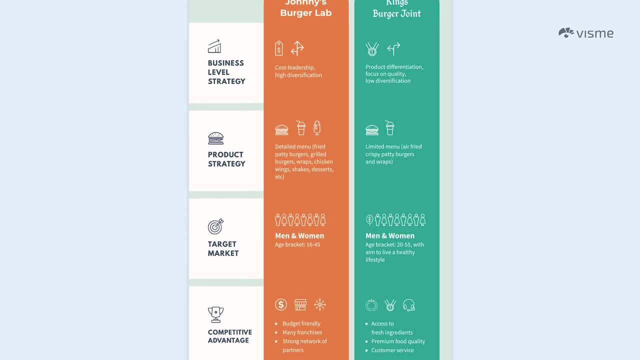 competitors. Compare your company with another one in the industry to see how they match up with one another. side by side. It can be eye-opening, sure, but take a hard look at the competition. It's crucial if you want to compete in the market. 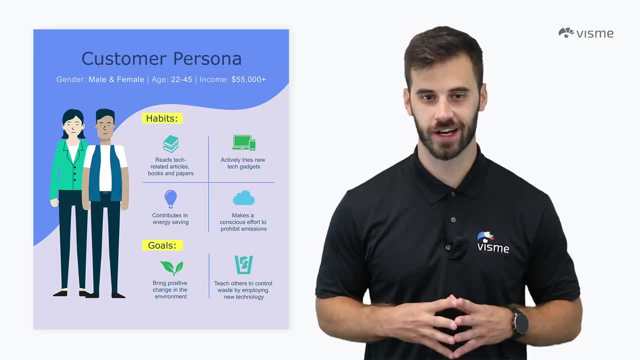 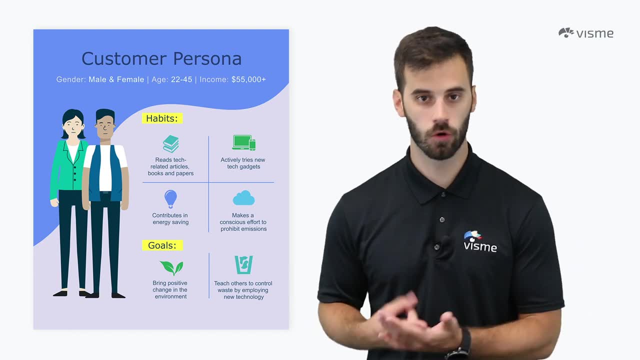 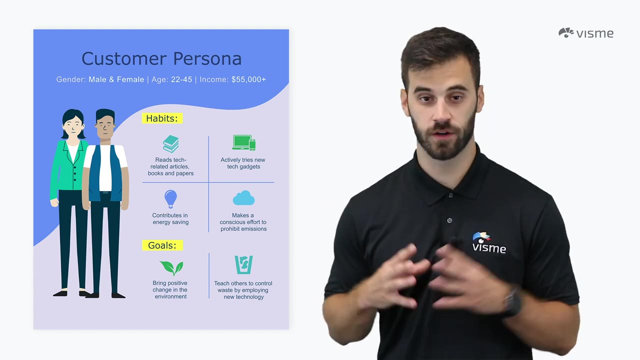 After identifying your competition, you must identify your target customer. This will allow you to create more informed and tailored marketing strategies. Build a person from scratch. How old are they? What's their income? What are their interests? What do they value? A template like this is perfect for putting that. 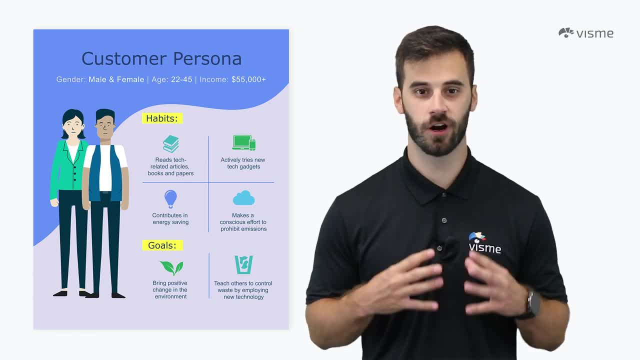 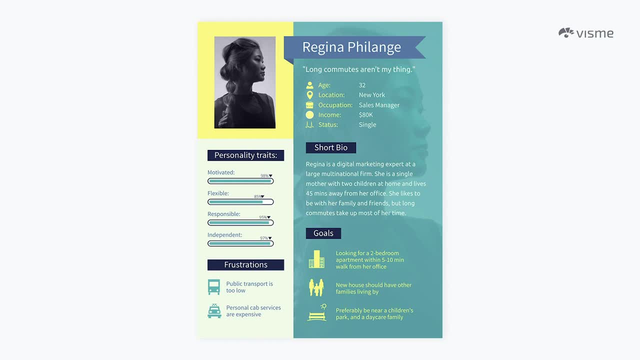 person you've built on paper and explaining him or her to your audience during a presentation or during a meeting, Or what's one way that's almost always used when someone wants to explain themselves for a job- Well, a resume, of course. This template more closely resembles an actual. 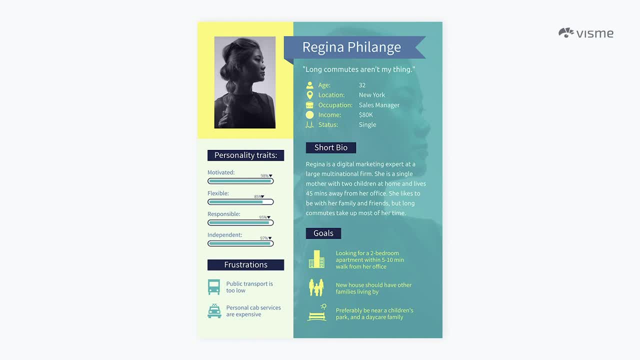 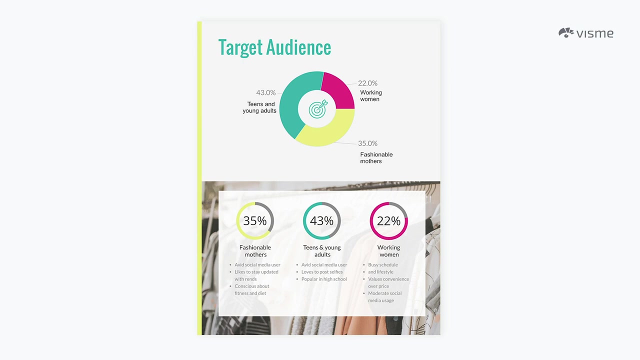 resume. It includes basic information, a photograph, personality traits, a bio, goals, frustrations. you can edit it however you see fit to describe your target audience. And if your target audience is a mixture of different people, try creating an infographic. with data widgets You can break down how much you. 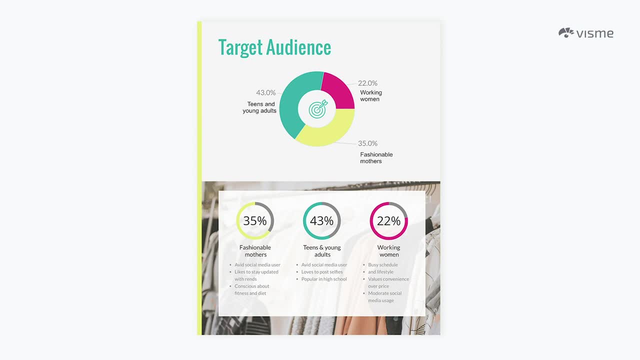 should cater to one group or the other. There's a number of different charts and graphs you can use to help, but this template went with pie charts to break down target customer percentages. It's easier to understand than if someone was trying to explain it without a visual. 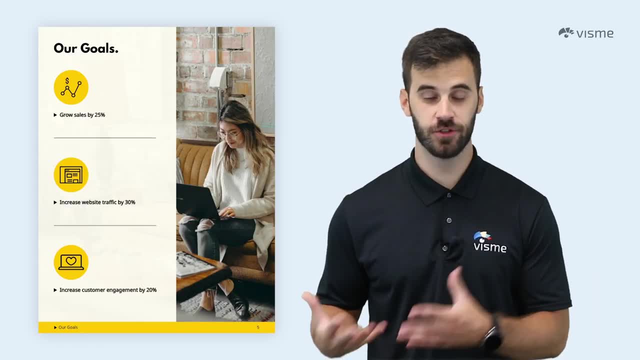 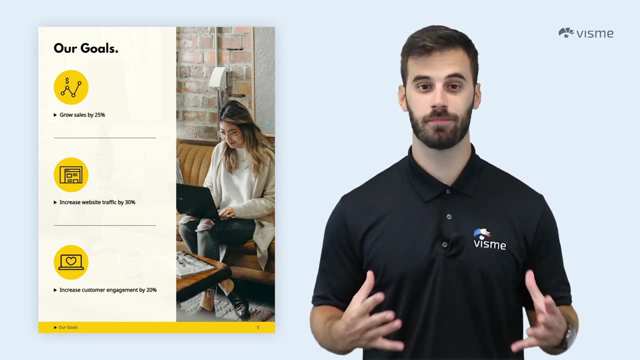 Okay, you've done your research. you know your audience. now it's time to outline your marketing goals. What are you hoping to achieve with your marketing plan? The most important thing to remember with this step is to be specific with actual numbers If you're hoping to achieve more. 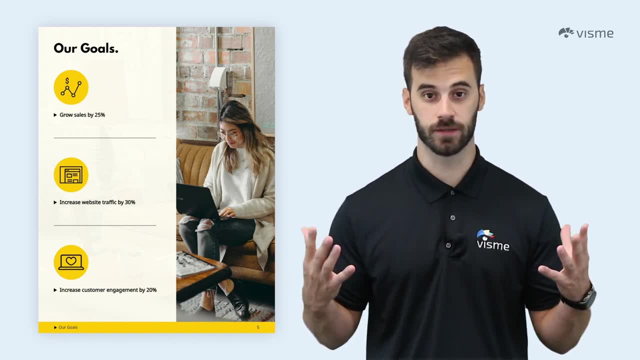 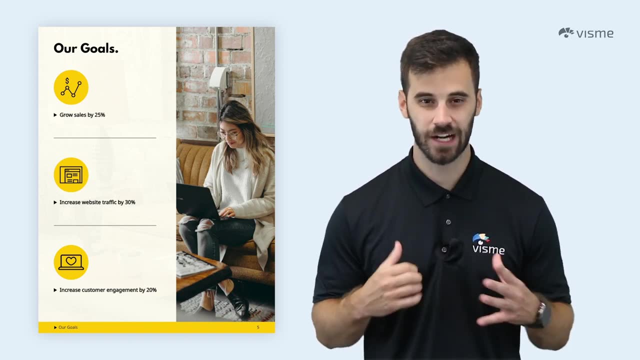 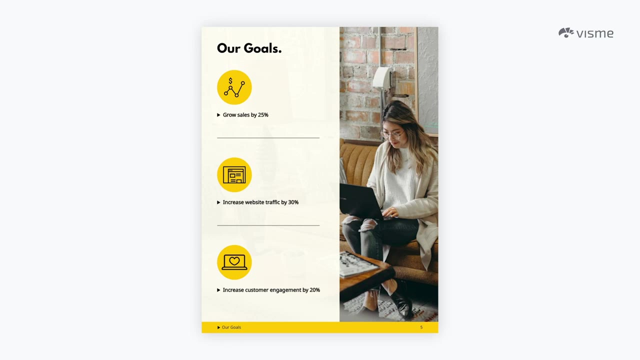 web traffic. don't just say the goal here is to increase web traffic. Say my goal is to increase traffic to our site by 30% within the next three months. You need a concrete goal, not a blanket statement. This template is simple, easy to digest and lays out specific goals. They're all measurable. 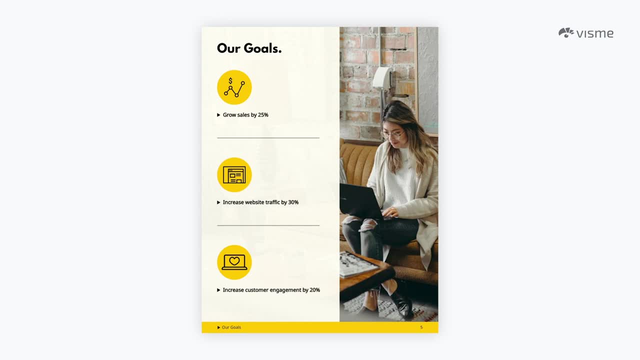 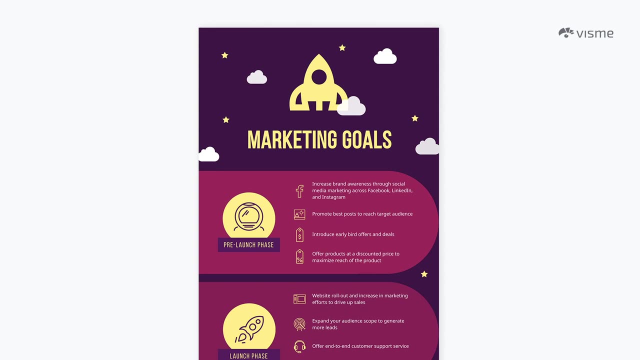 and clear. Following the progress towards the goals won't be difficult with how definitive they are And, as I mentioned, deadlines could be used as well. If that's the case, a template like this could be more fitting: In order for this company to accomplish a goal: these three phases. 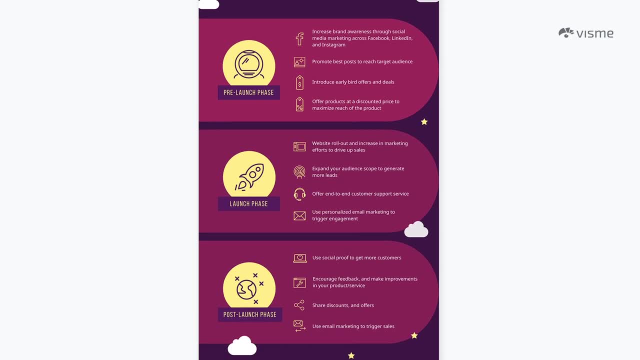 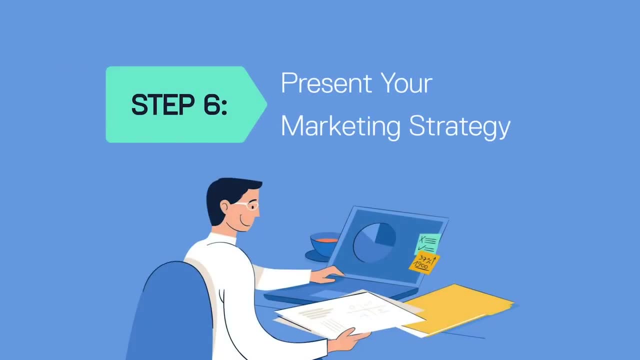 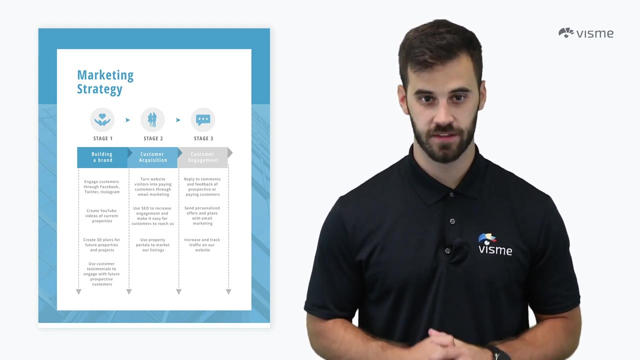 must be properly carried out. Marketing plans like this help viewers follow along, as they can refer back to them if they start to get off. Continuing off my last point, our sixth step is to lay out your marketing strategy from beginning to end. There's three details to write down and include with this step One: what to do. 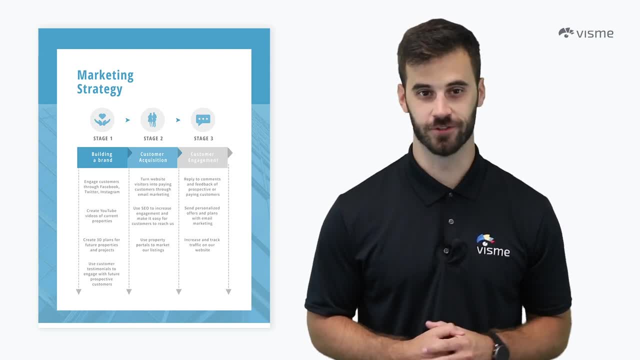 Two, how to do it And three, the channels to use. I highly recommend turning this into a visual so your team and audience can fully understand your thought process, To make it even easier for them turn your strategy into a series of phases or steps. 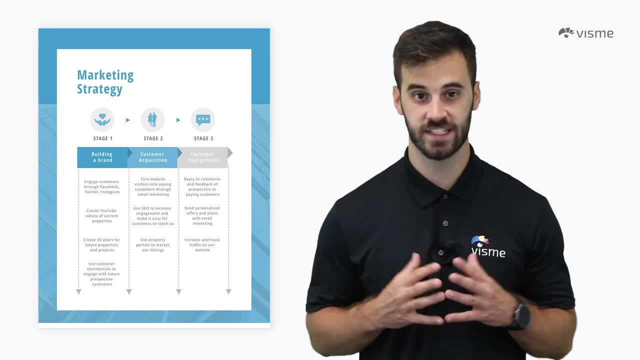 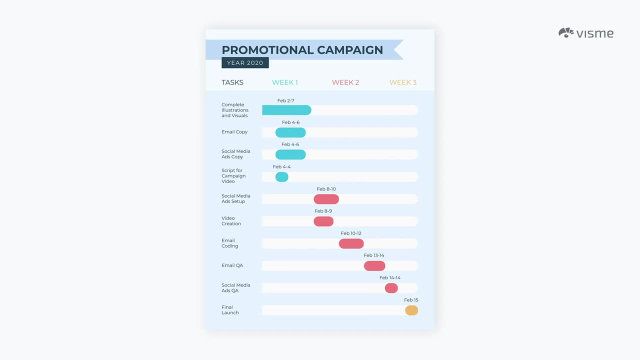 It could look something like this: clarifying what needs to be done in each step before moving on. Or, if you want more certain dates and deadlines, this template here could be even better. Specific dates are laid out from the first phase of the project to the launch. If you want to ensure. 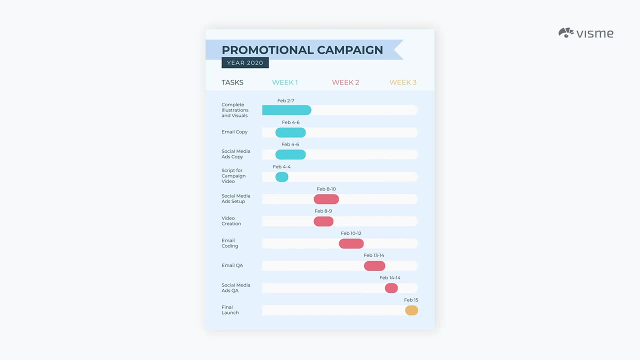 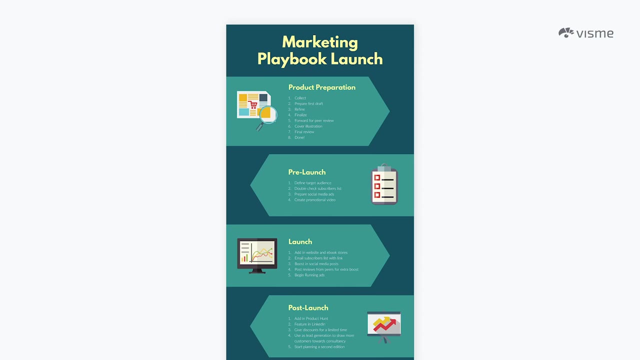 something is completed by a certain time. we highly recommend using this template. Infographics in general are wonderful for displaying information in a way that is easy to understand. People are much more likely to retain information compared with a visual rather than with text alone. Another template to consider is something: 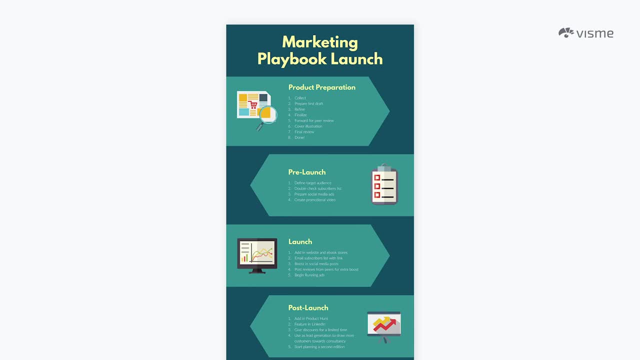 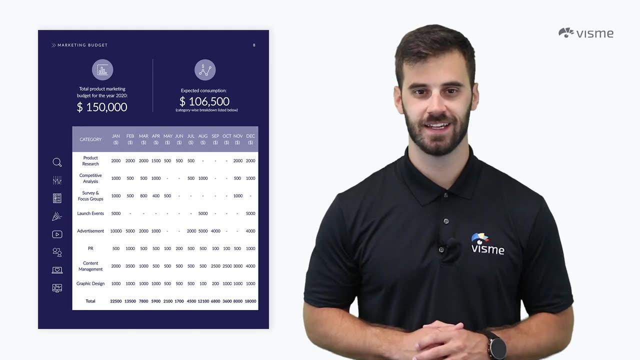 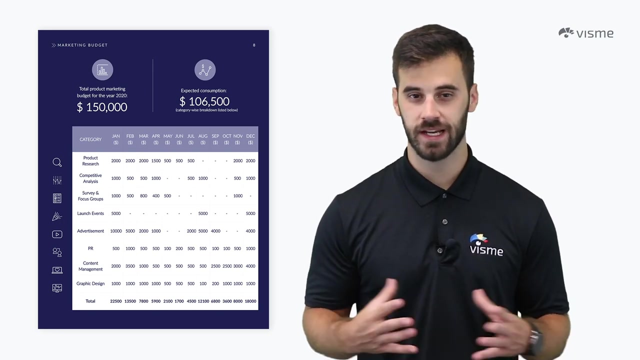 like this: Lay out all of your information in a detailed manner, leaving nothing to the imagination. Last but not least, detail the budget considerations for your plan. How much is it going to cost in order to reach your goal? It's important to be clear with this up front, at least. 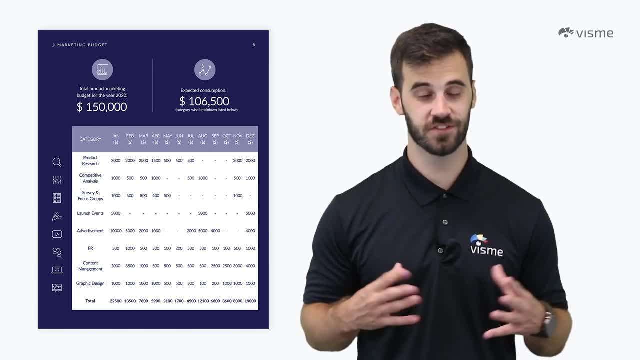 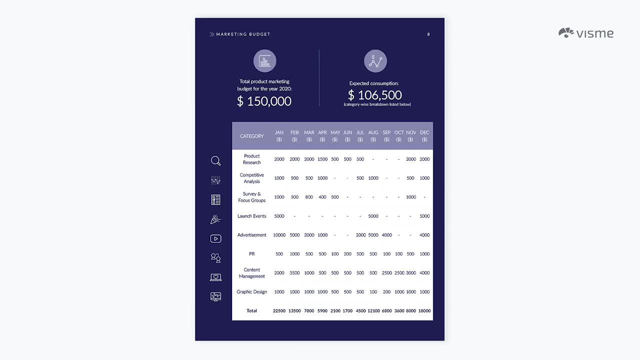 as best as you can. Marketing can be costly and there are often a lot of hidden expenses. This may be the most helpful template of all. It clearly lays out the cost to your company. Try to set a cap early on, so you have a goal to stay under from the jump. 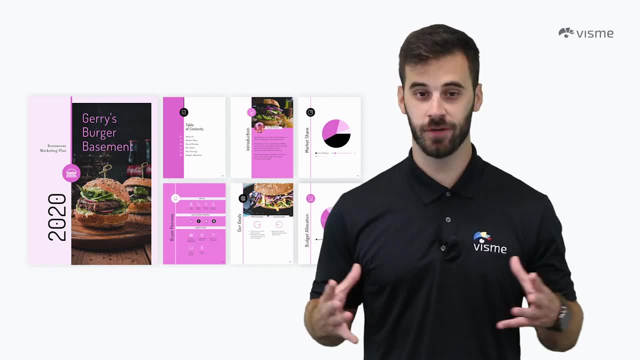 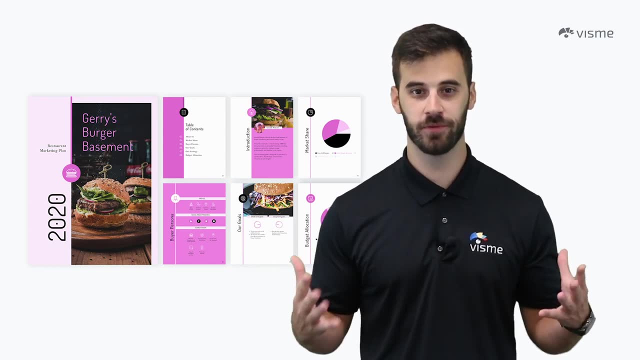 Okay, we've covered the steps for preparing your marketing plan. You should be able to put one together from start to finish, but I did want to share just a few more VisMe templates that may help you, depending on what industry you're in. 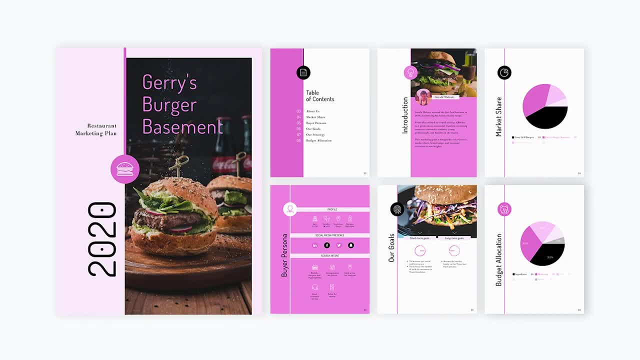 Business Templates. This restaurant marketing plan template is versatile for either massive chains or local eateries. You can replace the photos with your own and change the colors, just like with other templates, If you're in real estate and are part of a team, or even if you're operating your own. 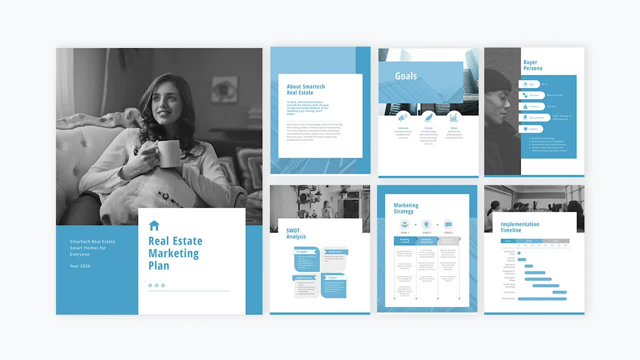 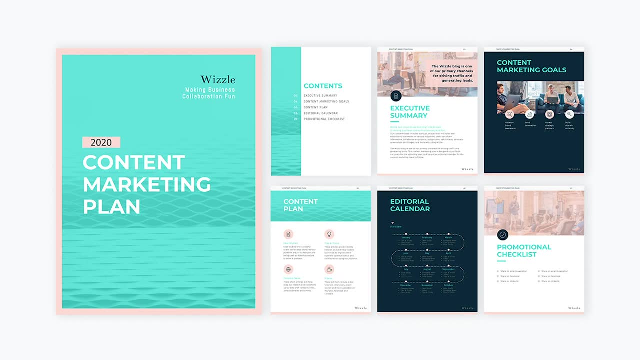 business. this template here can be useful. The SWOT analysis included makes it perfect for businesses focused on property marketing. Maybe you work for a SaaS or content company and you're looking to take your content to the next level. This template. 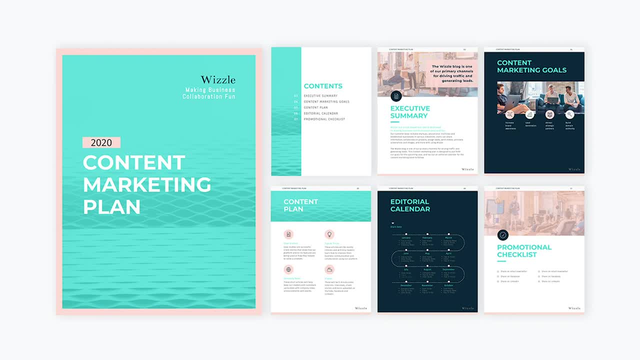 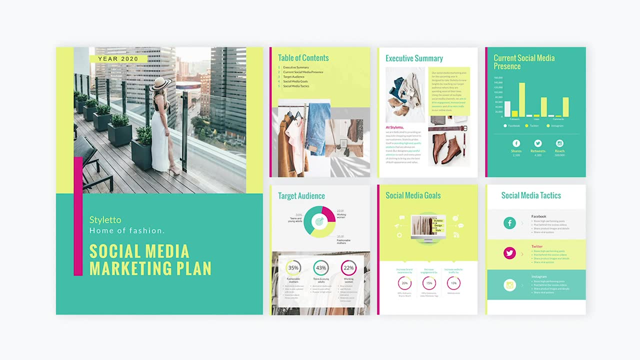 will help you organize your editorial calendar so you're able to reach your goals on time. Or what about social media? We all manage our own pages of some sort, and all businesses should have their own as well. Want more followers. This template can lay out.